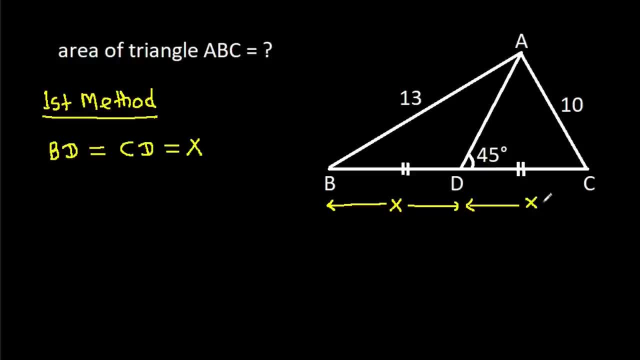 X and CD is X. And now, from point A, if we draw a perpendicular on BC, suppose this point is E and suppose AE is H, AE is H. And now inter angle: ADE. it is ADE. This angle is 90 degree, This angle is 45 degree. 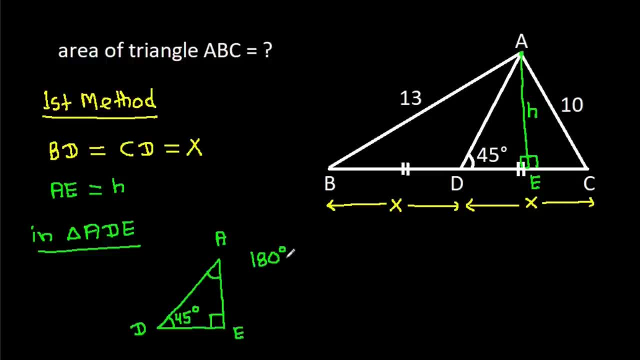 So this angle, it will be 180 degree minus 90 degree, minus 45 degree, That will be 45 degree. So it will be 45 degree And we have angle EAD is equal to angle EDA. That is 45 degree. So EA it will be equal to ED. 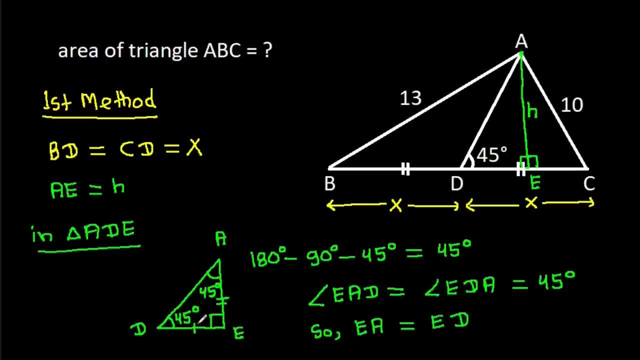 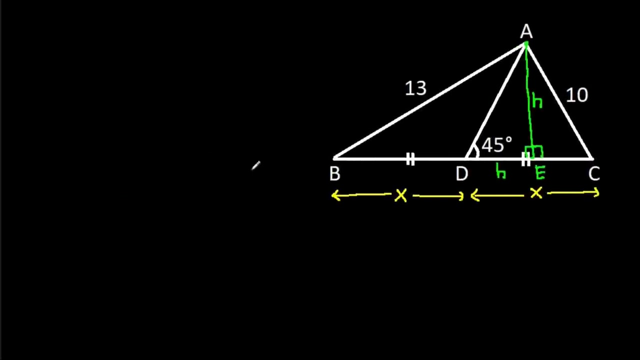 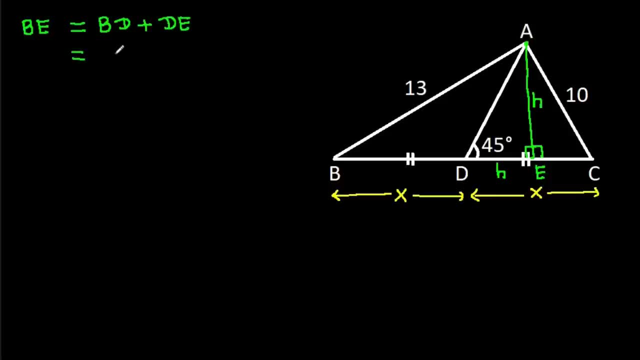 plus DE and BD is X plus DE is H, So BE it will be X plus H And CE it will be CD minus DE, and CD is X minus DE is H, So CE it is X minus H, And now interangle ABE it is: 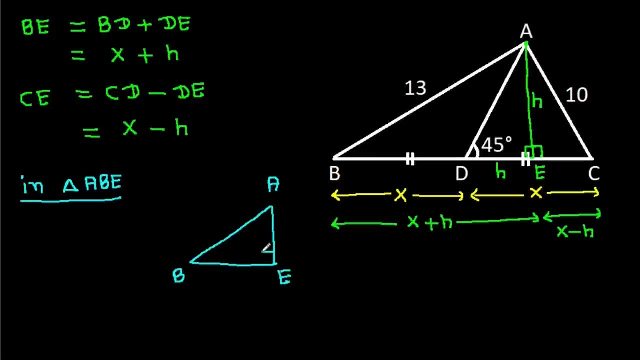 a, b, e. this angle is 90 degree. ae is h, be is x plus h and ab is 13. So ae square plus be square, it will be equal to ab square by Pythagoras theorem And ae is h square. 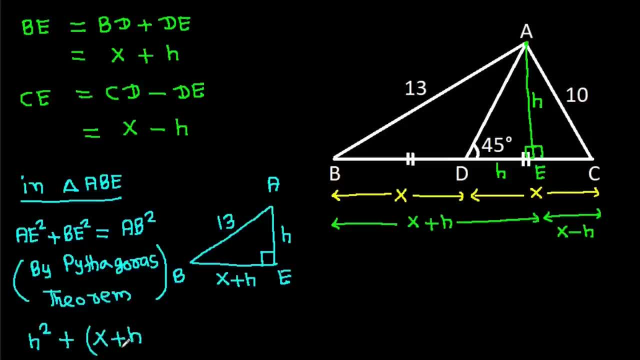 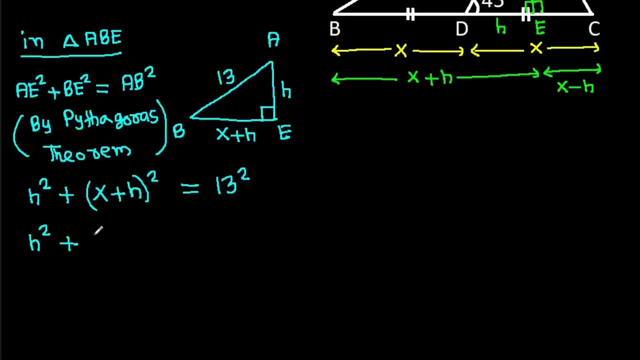 plus be is x plus h square. it is equal to ab square. ab is 13 square and it is h square plus. this will be x square plus h square plus 2xh. it is equal to 13 square is 169.. And h square plus h square, it is equal to 13 square plus. 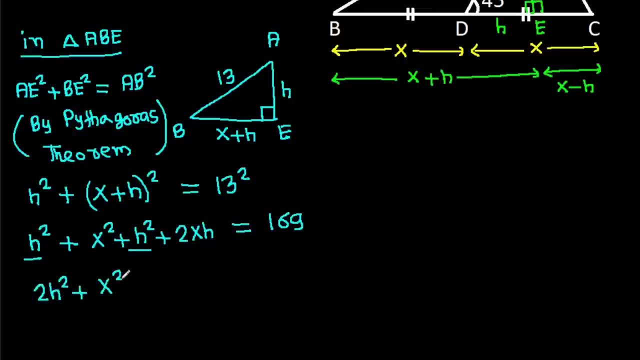 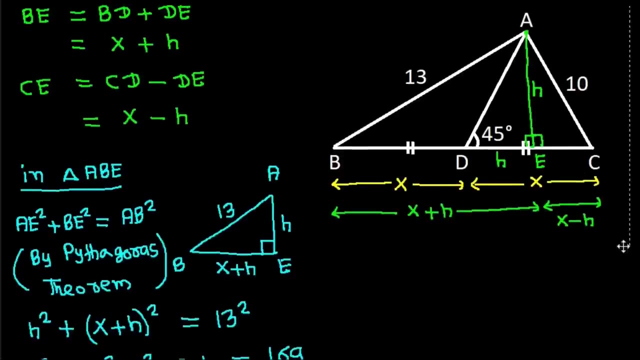 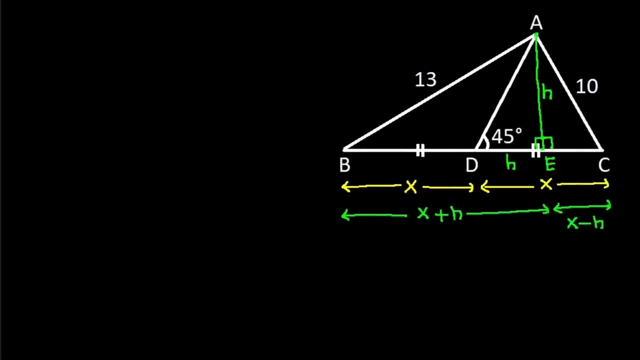 x square plus h square plus h square plus 2xh, it will be 2: h square plus x square plus 2xh, it is 169.. Suppose it is equation 1, and now inter angle A C E, It is A C E. This angle is 90 degree. 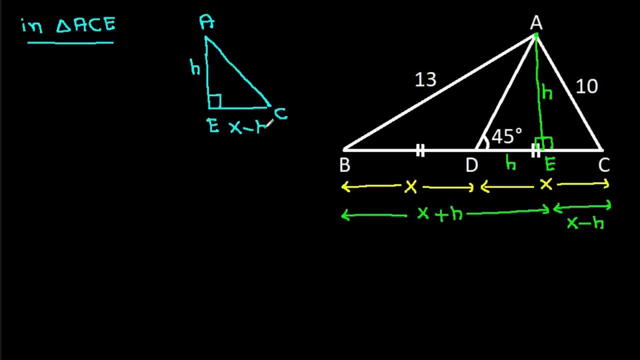 A E is H, C E is X minus H And A C is 10.. So A E square plus C E square, It will be A C E square by Pythagoras theorem, And A? E is H E square plus C? E is X minus H E square. 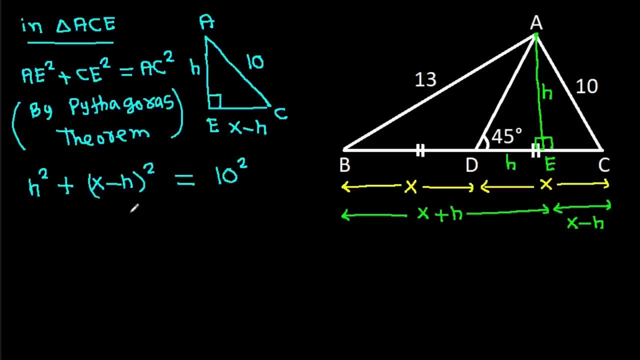 It is equal to A. C is 10, E square, And it is H E square plus X minus H E square. It will be X E square plus H E square minus 2X H. It is equal to 10, E square is 100.. 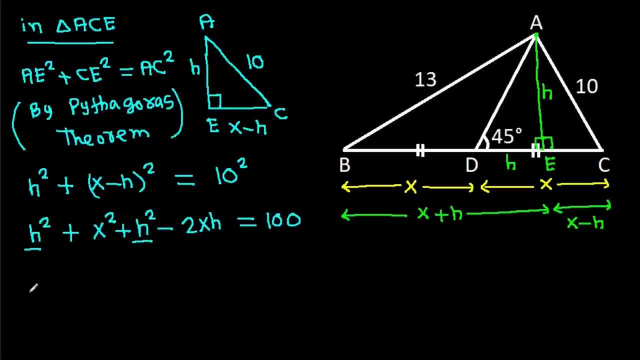 And H? E square plus H E square, It will be A C E square. by Pythagoras theorem, It will be 2X S square plus X S square minus 2X H, It is 100.. 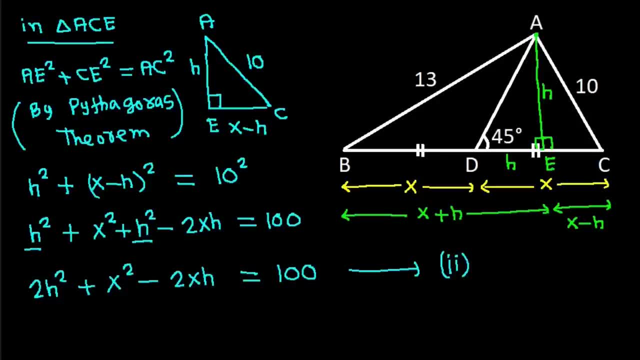 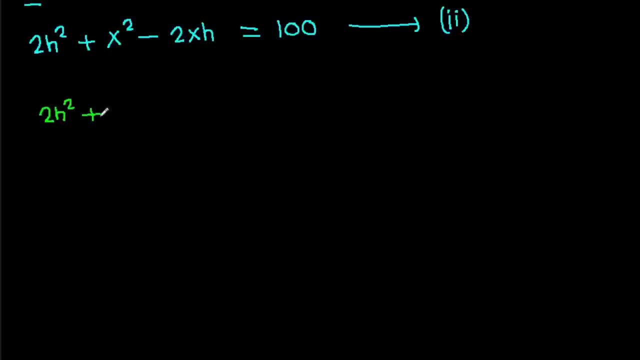 Suppose it is equation 2. And we have 2X S square plus X S square plus 2X H is 169.. It is equation 1. And 2X S square plus X S square minus 2X H is 100.. 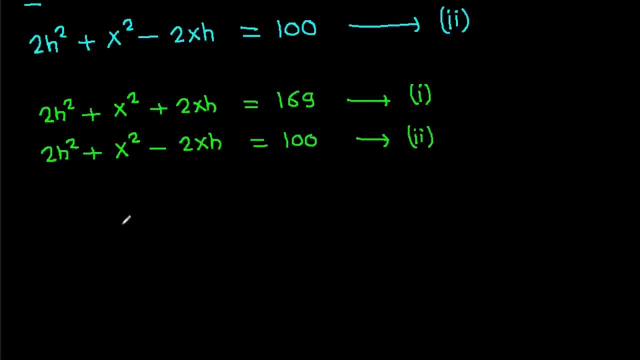 It is equation 2.. And if we subtract equation 2 from equation 1, equation 1 minus equation 2, then 2X S square plus X S square plus 2X H Minus 2X S square plus X S square minus 2X H. 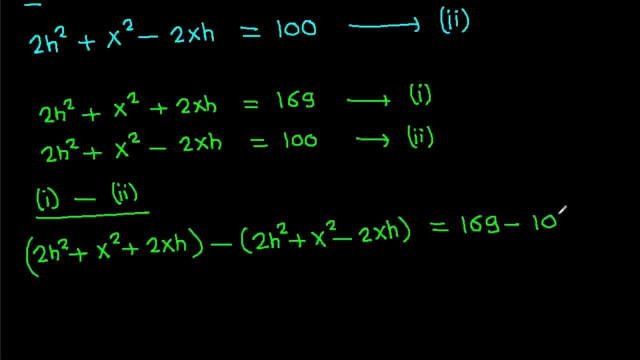 It will be 169 minus 100.. And 2X S square will get cancelled. X S square will get cancelled. So it is 2X S Minus 2X S square, plus X S square minus 2X H. 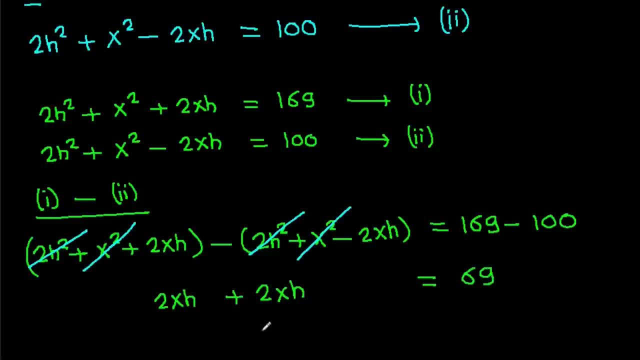 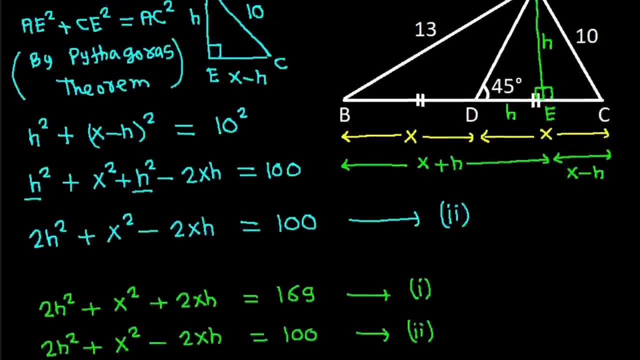 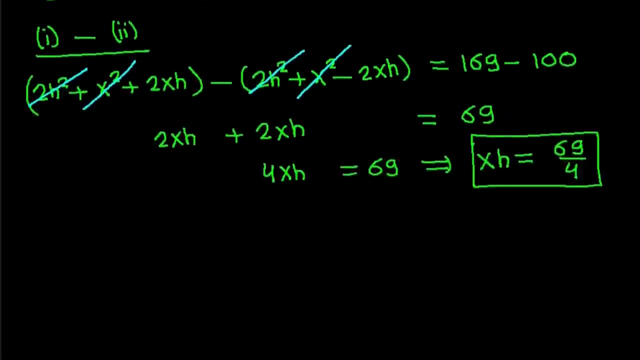 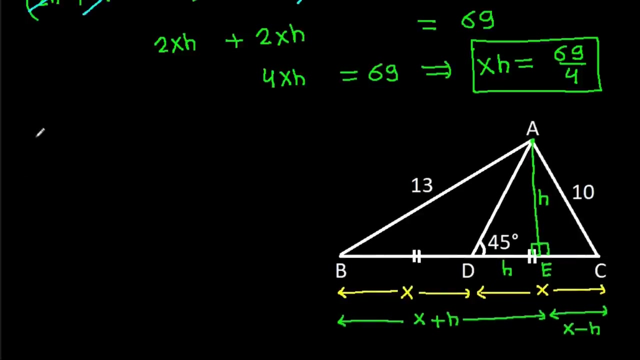 It is equal to 69. And 4X S is 69. That means X S, it will be 69 by 4.. And Now area of ABC. it will be 1 by 2 times. base is BC and height is AE, and it is 1. 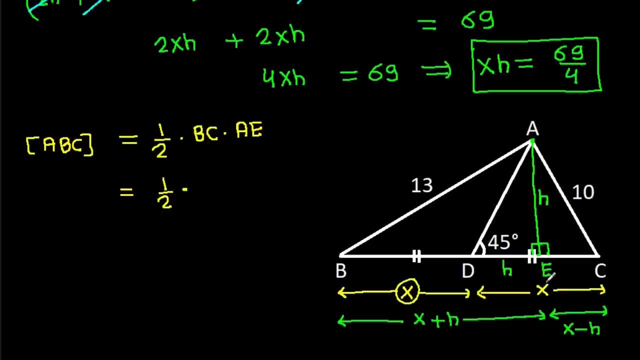 by 2 times BC is X plus X. that will be 2 X times AE is H and 2 will get cancelled. so it is X, H and X. H is 69 by 4. so area of ABC it will be 69 by 4 and 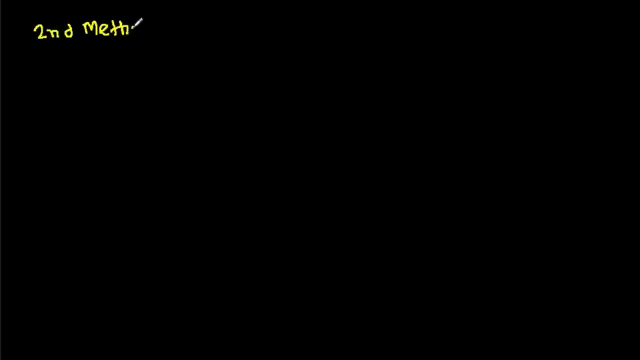 the second method occurred at area of films. right now in HAM we have bbr, bcdh, bd,1 and bd,3. we have series of lines also Na na, 0.02, and so this we can find this factsample substantiating. 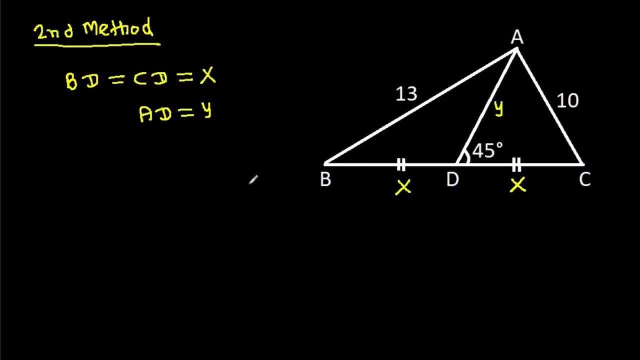 since the number of lines spinning till the previous order. so we have ±h by 2x, So this is also possible. Next you can see here: 2019.. and D: this angle is 45 degree, so this angle, it will be 180 degree minus 45 degree that. 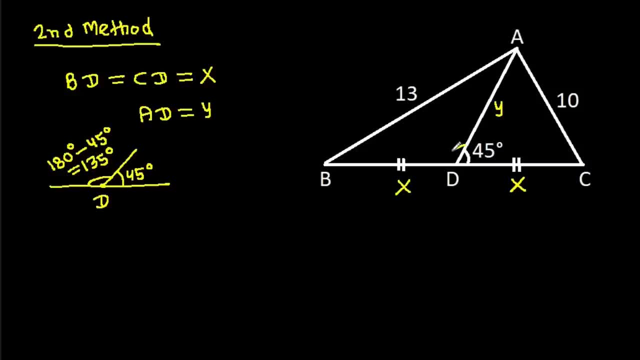 will be 135 degree. so this angle, it will be 135 degree. And now in any triangle, ABC, if AB is A, AC is B, BC is C and this angle is theta, then cos theta it is A square minus B square minus C, square by 2AB. 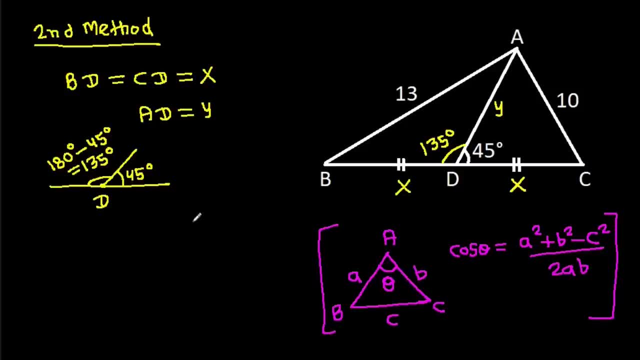 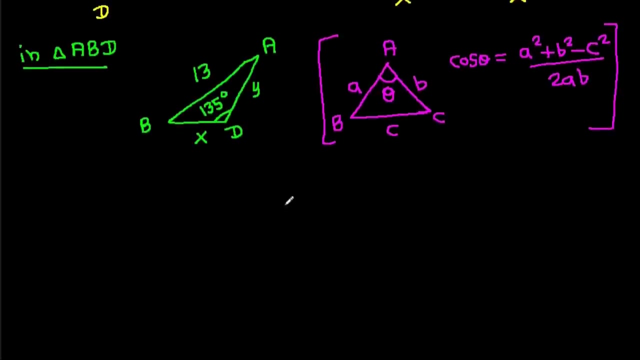 so. So here inter angle ABD it is ABD, AB is 13,, BD is X, AD is Y and this angle is 135 degree. So cos 135 degree it will be BD square plus AD square, minus AB square by 2 times BD times AD and cos 135 degree it is minus 1 by square root of 2.. 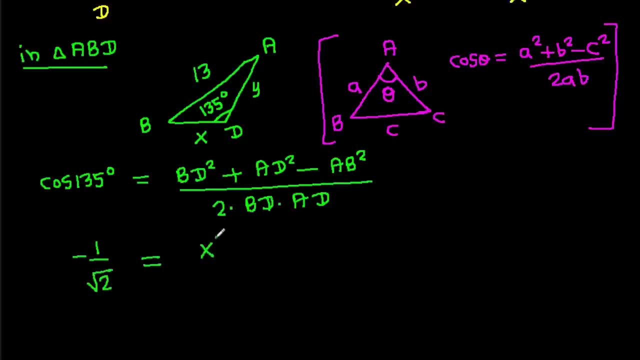 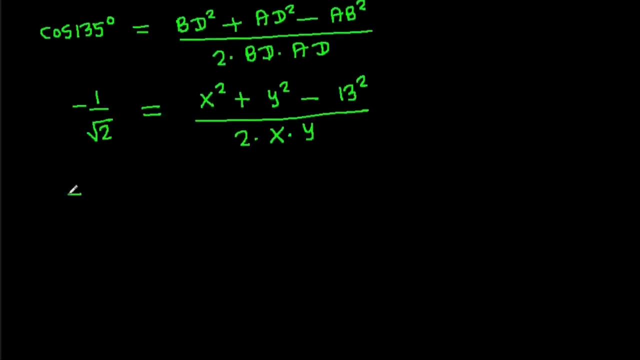 It is equal to: BD is X. A square plus AD is Y. a square minus AB is 13,. a square by 2 times BD is X, AD is Y, And if we cross, multiply then minus 2XY by a square root of 2, it will be X square plus. 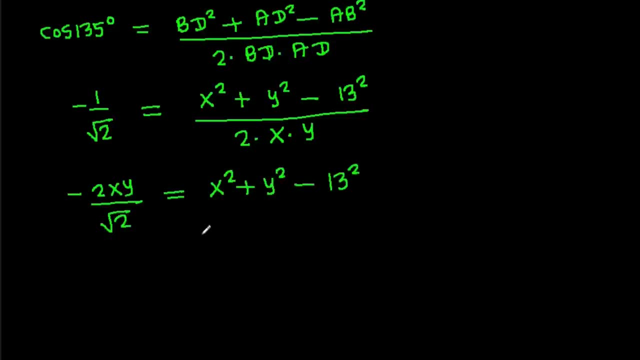 Y square minus 13 a square and a square root of 2 times a square root of 2 is 2.. So minus a square root of 2, x, y, it is x square plus y square minus 13 square is 169.. Suppose: 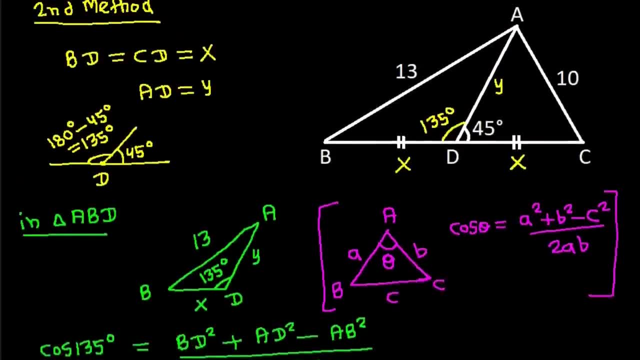 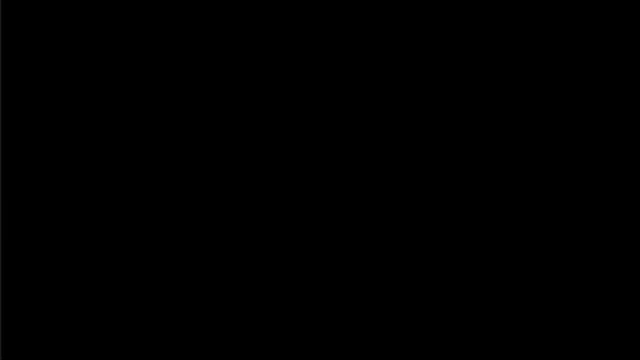 it is equation 1. and now inter angle a, c, d, it is a, c, d, c, d is x, a, c, d, c, d is x, a, c, d, c, d is x. a, c is 10, a, d is y, and this angle is 45 degree. So, cos 45 degree, it will be c, d, a square. 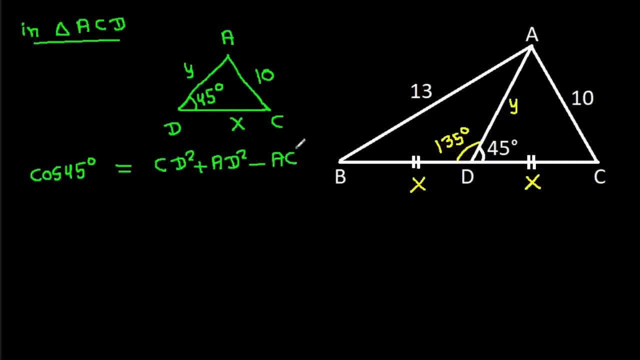 plus a d a square. minus a c a square. by 2 times c, d, times a d and cos 45 degree, it is 1. by a square root of 2 it is equal to: c. d is x a square. plus a. d is y a square. minus a. c is 10 a square. 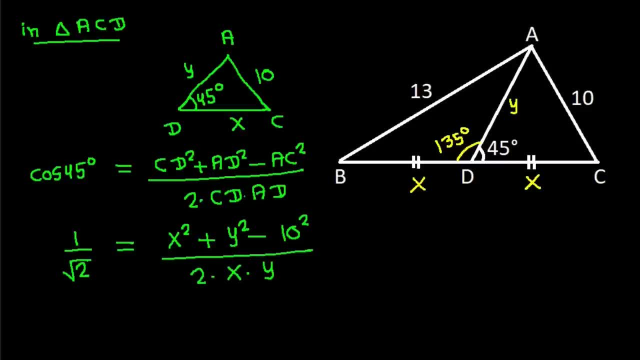 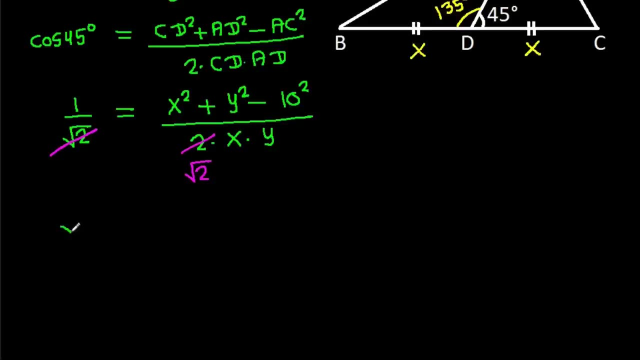 by 2 times x, times y, and a square root of 2 times a. square root of 2 is 2 and if we cross multiply, then a square root of 2 x y, it will be x, a square, plus y, a square, minus 10, a square and a. 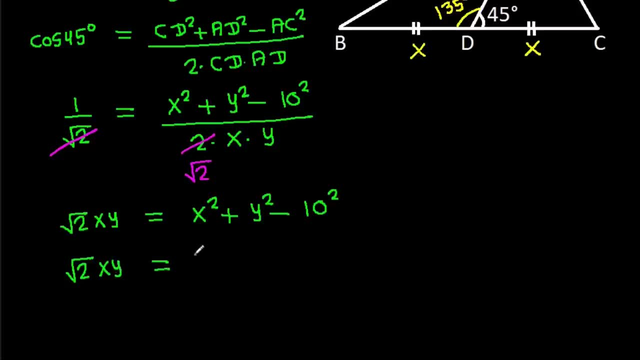 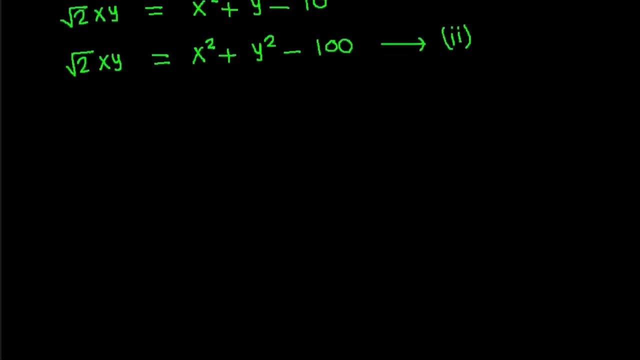 square root of 2 x, y. it is x a square plus y a square minus 10, a square is 100.. Suppose it is equation 2.. Suppose it is equation 2.. So we have minus: a square root of 2 xy is x square plus y square minus 169.. 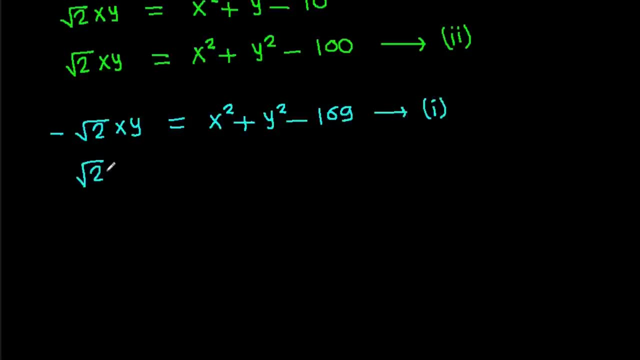 It is equation 1 and a square root of 2 xy. it is x square plus y square minus 100.. It is equation 2.. And if we subtract equation 1 from equation 2, equation 2 minus equation 1, then a square. 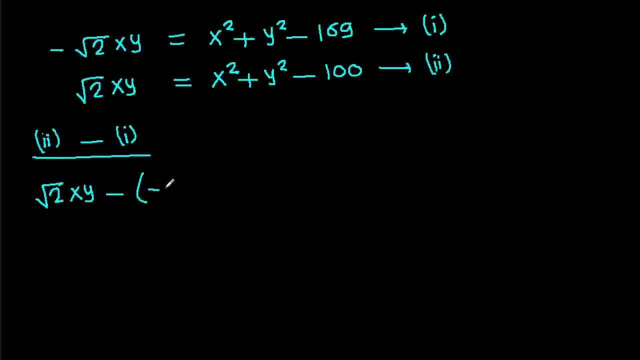 root of 2 xy, minus minus a square root of 2 xy, it will be equal to x square plus y square minus xy. So we have minus a square minus 100, minus x square, plus y square minus 169 and x square will get cancelled, y square will get cancelled and it is a square root of 2 xy plus a square. 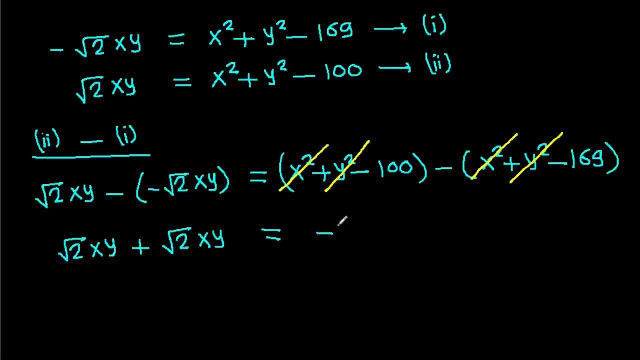 root of 2 xy is x square plus y square minus 169.. This equation is equal to minus 100 plus 100, 69, and it is 2 times a square root of 2. xy is 69.. So xy it will be 69 by 2 times a square root of 2.. 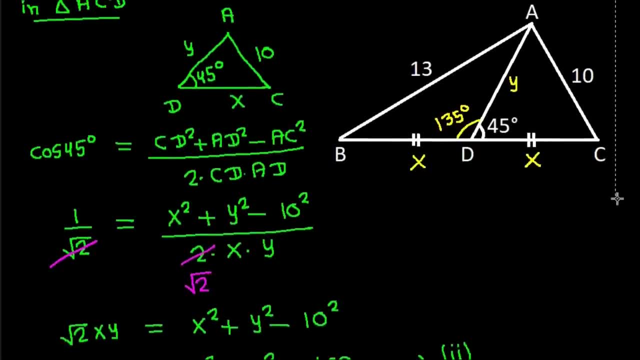 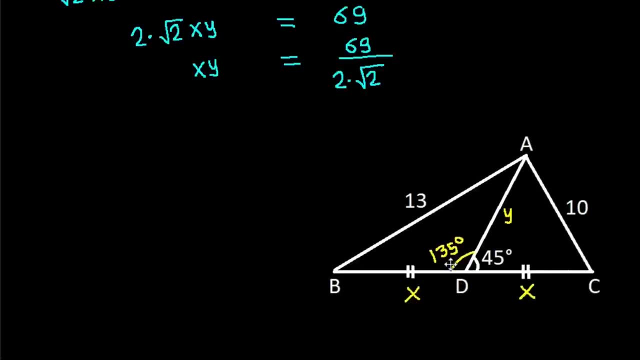 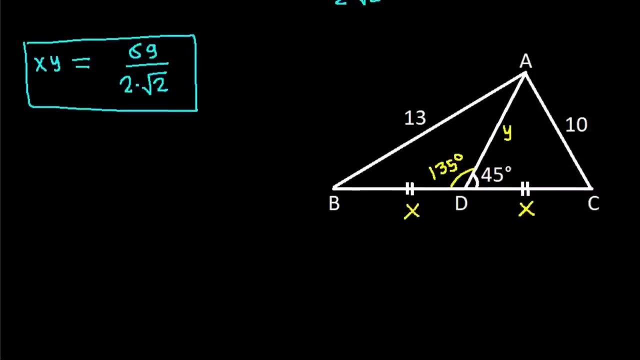 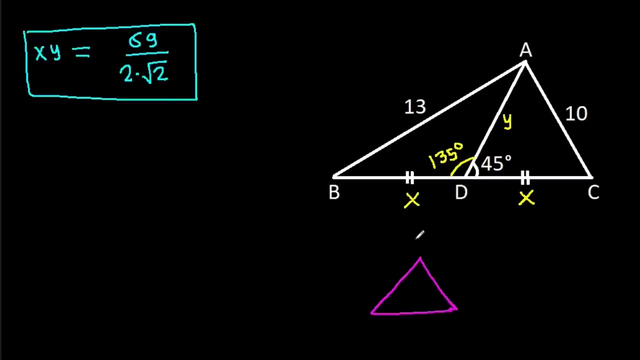 And xy, it is 169 by 2 times a square root of 2. xy, We get: xy is 69 by 2 times s square root of 2.. And now in anisotropic angle, A, B, C. if AB is A, AC is B and this angle is theta, then 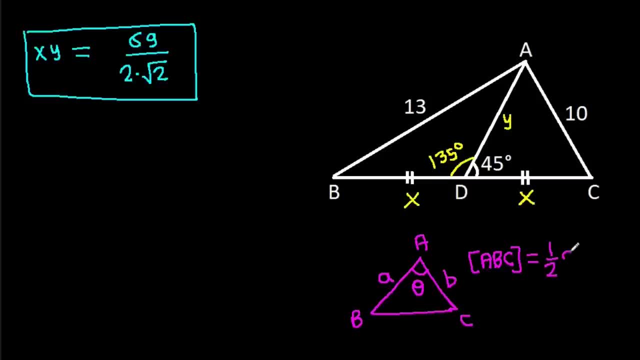 area of ABC it is 1 by 2, AB sin theta. So here area of ABC it will be area of ABD plus area of ACD and inter angle ABD. BD is X, AD is Y and this angle is 135 degree. So area of ABD it will be 1 by 2, XY sin 135. 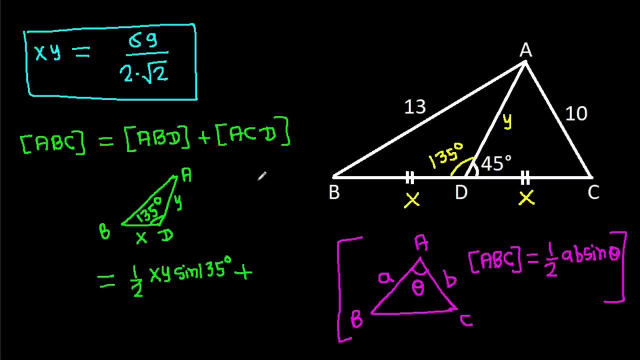 degree plus and inter angle ACD. this angle is 45 degree, AD is Y, CD is is x. So area of ACD it will be 1 by 2 xy sin 45 degree and it is 1 by 2 times xy is. 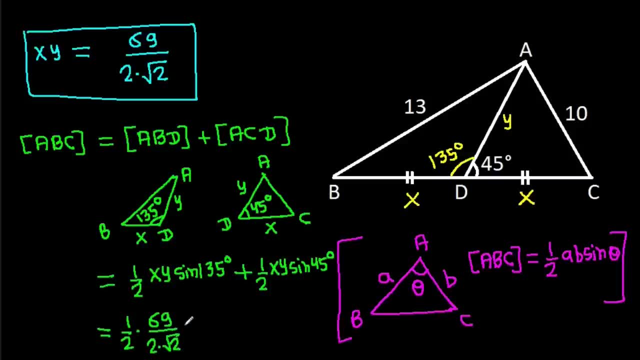 69 by 2 times square root of 2 times sin 135 degree, it is 1 by square root of 2 plus 1 by 2 times xy is 69 by 2 times square root of 2 times sin 45 degree. it is 1 by square root of 2.